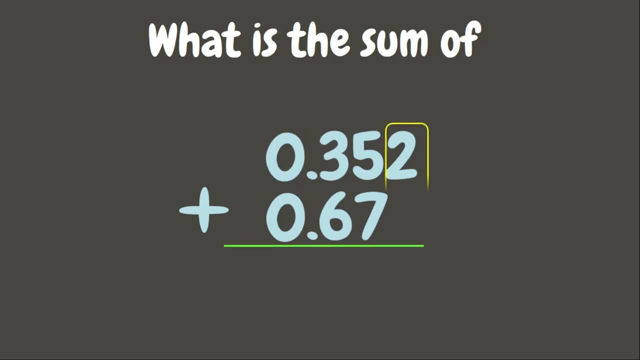 Now, let's add from right to left. Since there is an empty place value, we are going to put zero. 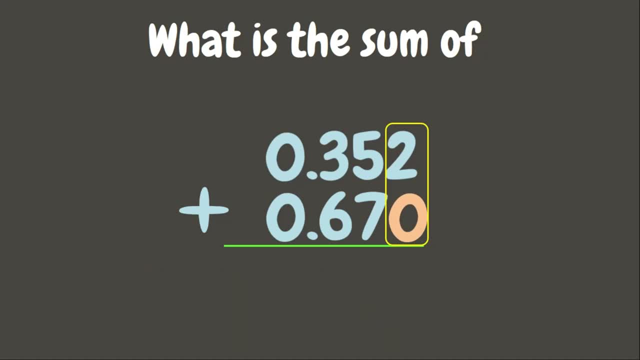 We are going to write the decimal with more of all the themselves. So, to make for 98 hundredths, let's add 503 hundredths and 78. The decimal number didn't get went together. 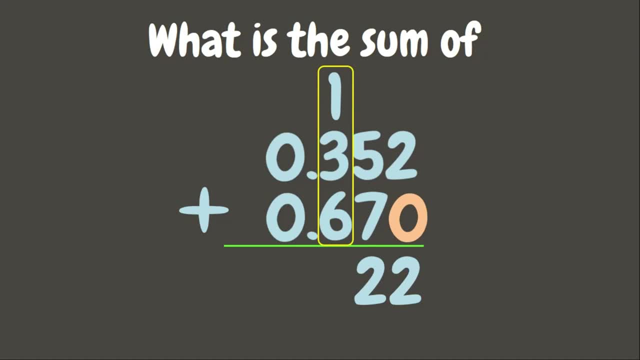 So what did we write? We wrote 82息 problem. The decimal plus zero is 2. And then, 5 plus� droit plus 7 is 12. 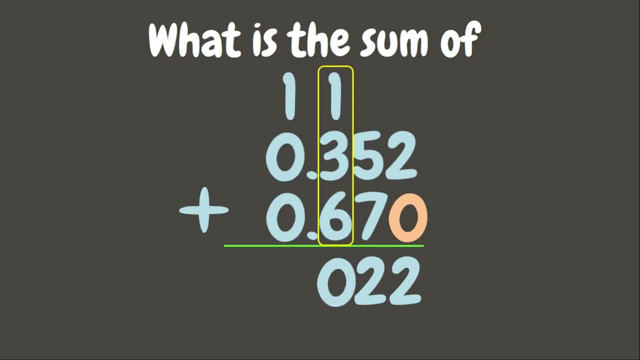 Write 2 and carry through one to the next place value. 1 plus 3 plus 6 that is 7藏 January. That is in-between these numbers.akat 7,7 and 8 in-between 마지막 place numbers. Okay. So, count when to add and stop. And then, 19% is 10% and 8 percent in combined. Write two to one. We add 1 and carry through 0 and accordingly 1.2. to the next place value put the decimal point a line from above and then 1 plus 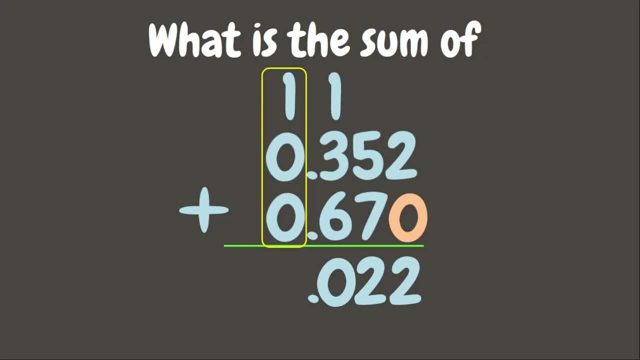 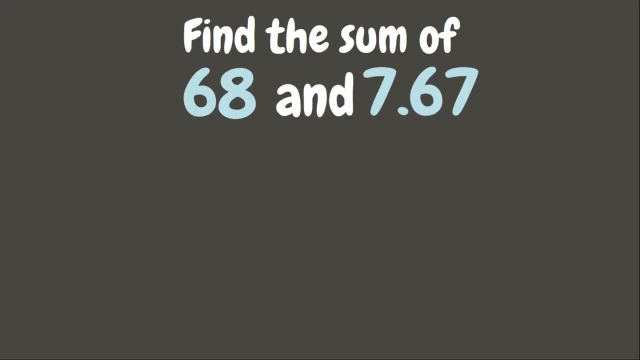 0 plus 0 is 1 our answer is 1 and 22 hundreds find the sum of 68 and 7 and 67 hundreds again when we are looking for the sum we are going to add you might be wondering where is the decimal point of a whole number the decimal point of whole numbers are found at the end of the whole number now let us align them 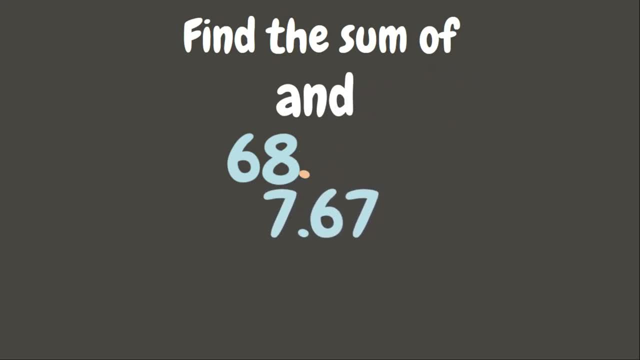 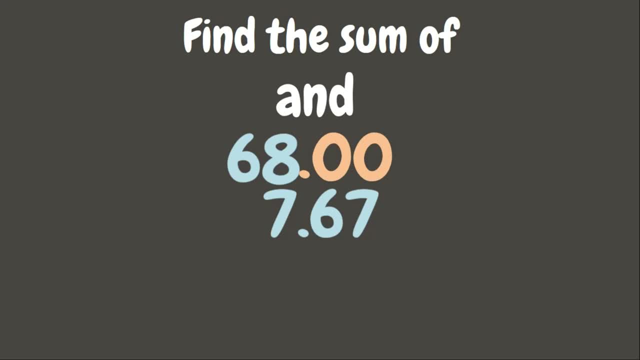 to the empty place values there now let us add 0 plus 7 is 7 0 plus 6 is 6 write decimal point a line from the decimal points above 8 plus 7 is 15 right 5 carry 1 to the next place value 1 plus 6 is 7 our answer is 75 and 67 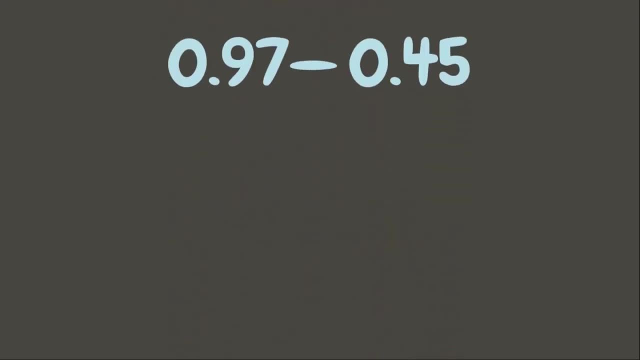 hundreds great job now let us try subtraction versus we need to align them vertically again make sure the decimal points and digits with similar place values are aligned now let us subtract 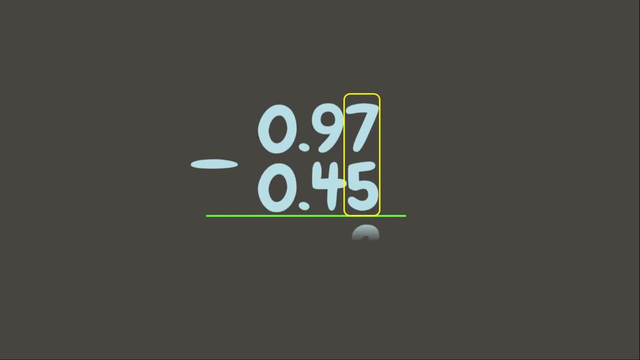 7 minus 5 is 2 9 minus 4 is 5 let us put the decimal point a line from the decimal points above and then 0 minus 0 is 0 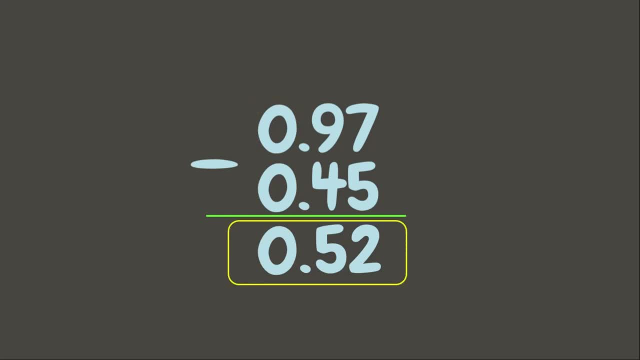 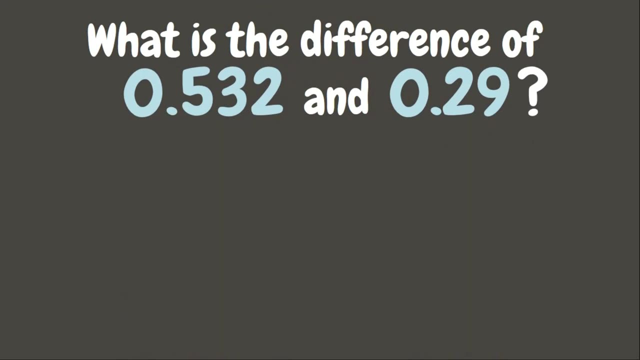 answer is 5200 they don't have another one what is the difference of 532000 and 29 hundreds if we are looking for the difference we need to subtract first let's align them vertically make sure again the 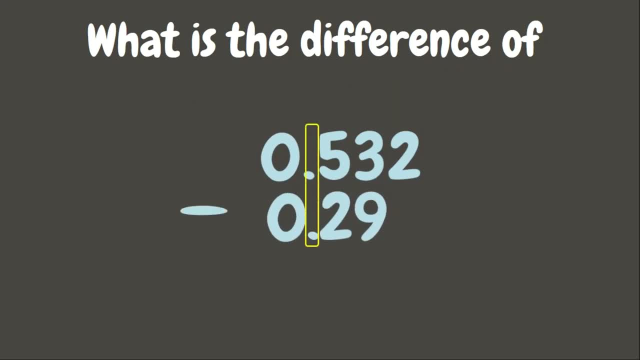 decimal points are aligned and they should be everything but you think proper tract itbreaker zone temperatura and ocean horizon we are not interested in water shall that's fine over here make sure Prem whatever number and what is your line let us subtract from right to left since there is an empty place value let's put zero 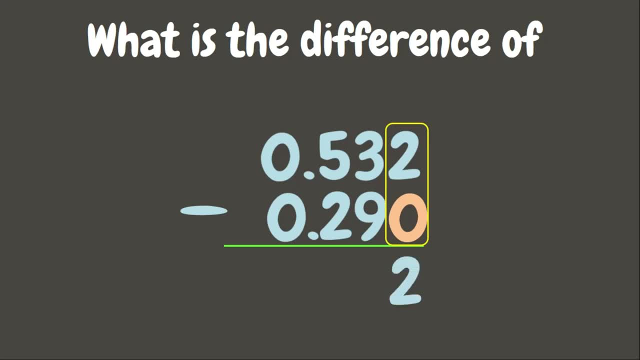 two minus zero is two three minus nine is cannot be we need to borrow from the next place value which is five let us borrow one from five five will be four and three will be thirteen thirteen minus nine is four next four minus two is two right 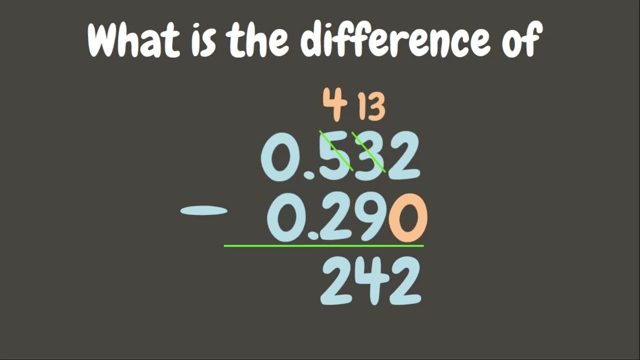 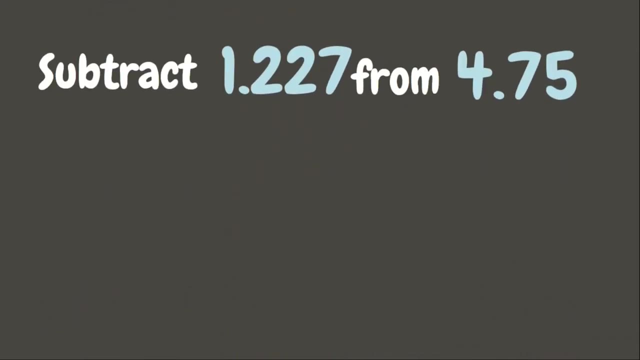 the decimal point a line from the decimal points above and then zero minus zero is zero our answer is 242 thousands let's have another example subtract 1 and 227 thousands from 4 and 75 hundreds